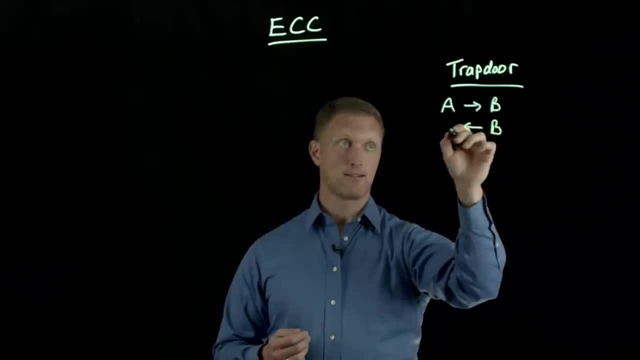 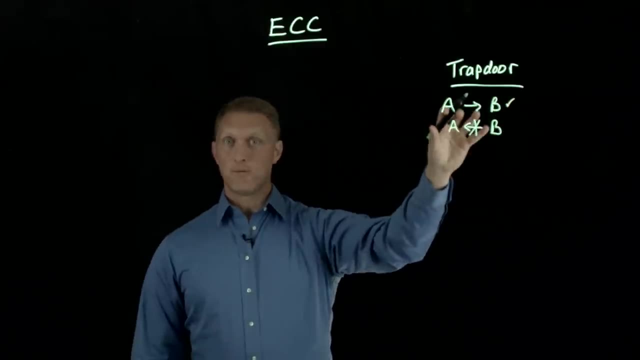 with the other value, say, start with B and then you want to get back to A, then it's very, very difficult to do that. So I'll put an X over that. I'll put a little check mark by that guy. All right, So again, trapdoor function. it's very easy to go one direction. 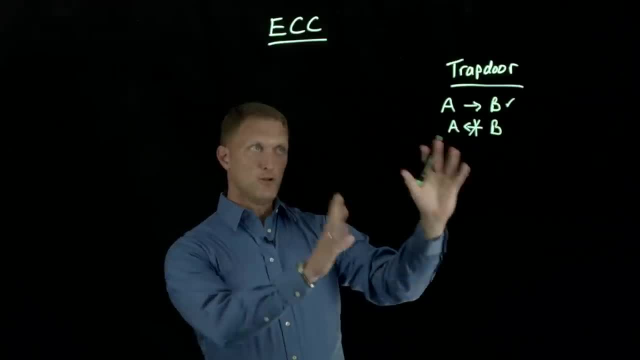 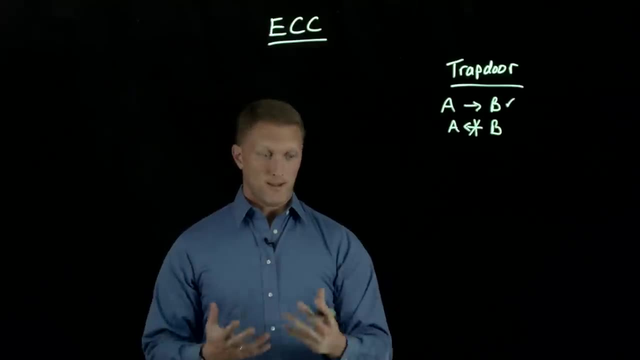 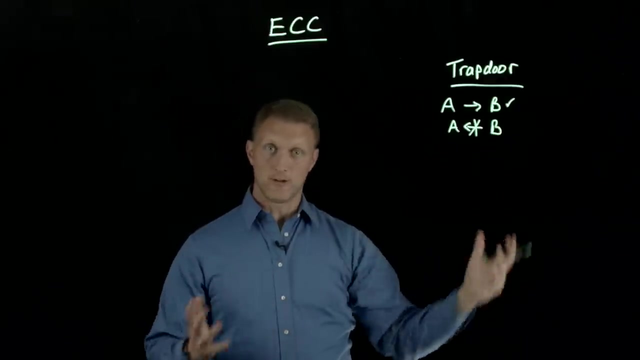 It's very difficult to go the other direction, And so, using that, and using that in the sense of a public key crypto system, you need some sort of a mathematical function, mathematical foundation, whereby you have a good trapdoor function to use for that public key crypto. 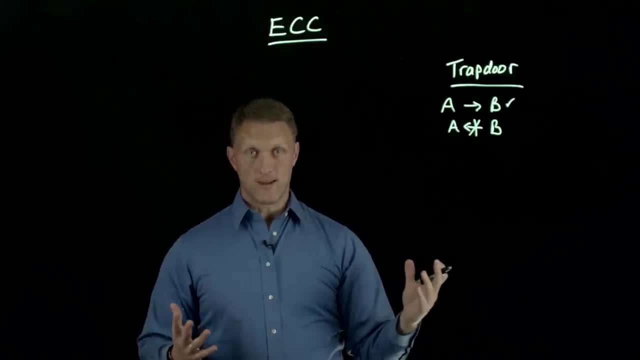 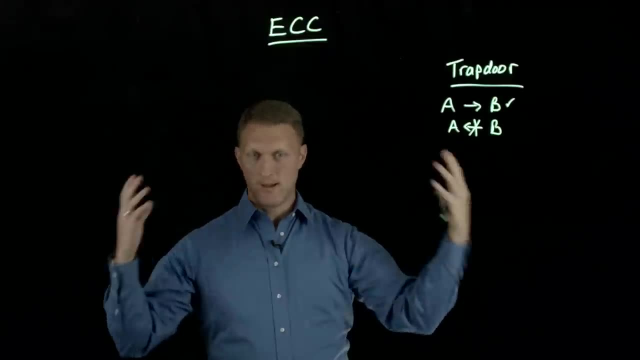 system, One that's used extensively today, is RSA, and it's based on prime number factorization, where you take two random prime numbers, you multiply them together, you get this really big prime number, and then the issue is: multiplying those together is very 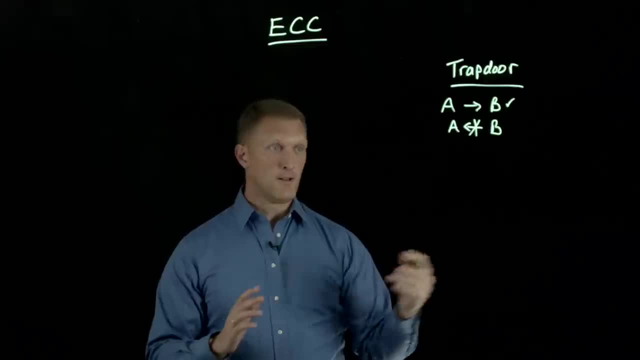 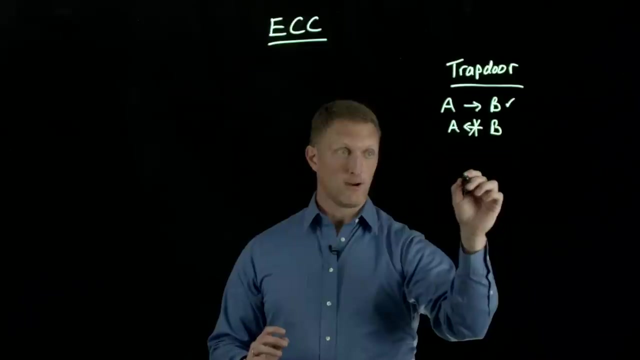 easy, which that's kind of that A to B level, But then to factor those out coming back from B to A is very difficult. That's kind of the really basic fundamentals of RSA and why it works so well today. One quick thing that I'll put on elliptic curve and RSA. I'll put ECC versus RSA. 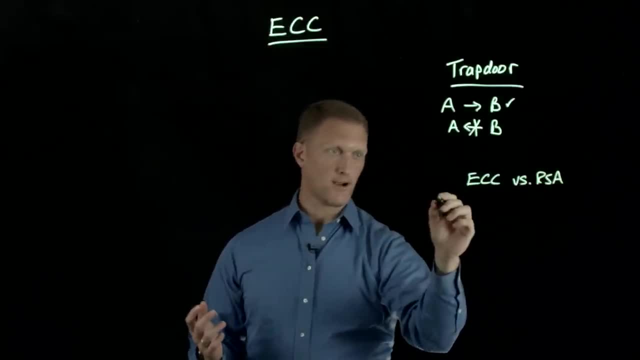 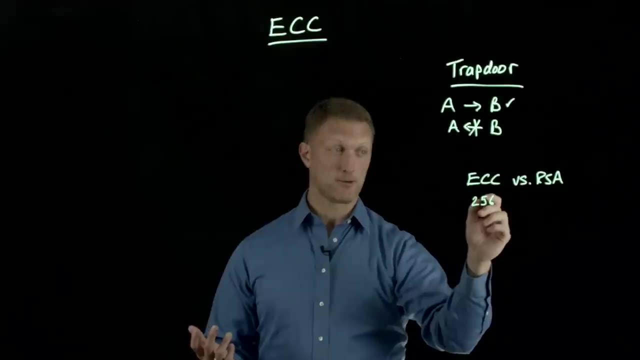 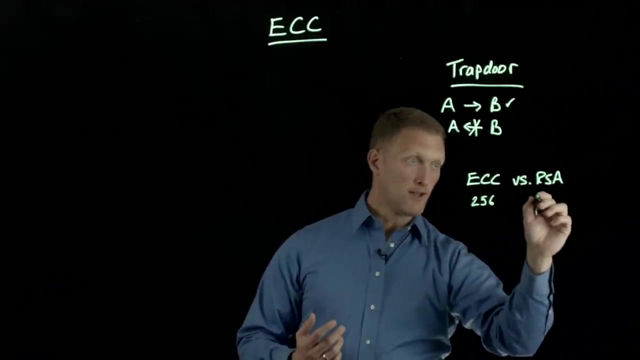 here And so with a key size in elliptic curve cryptography. if I were going to put, let's say, we talk about- a 256-bit key size in elliptic curve cryptography, in order to achieve that same level of security using an RSA key size, you would need a 3,072-bit key, And so you can start to see that. 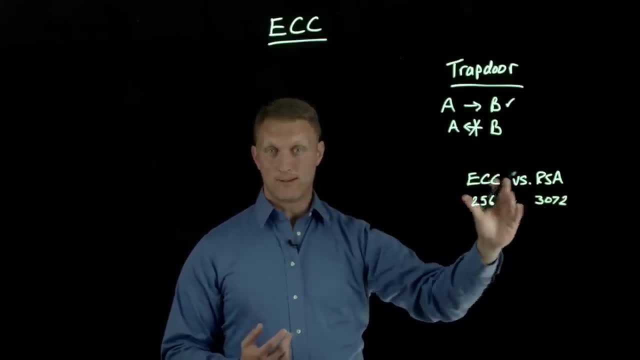 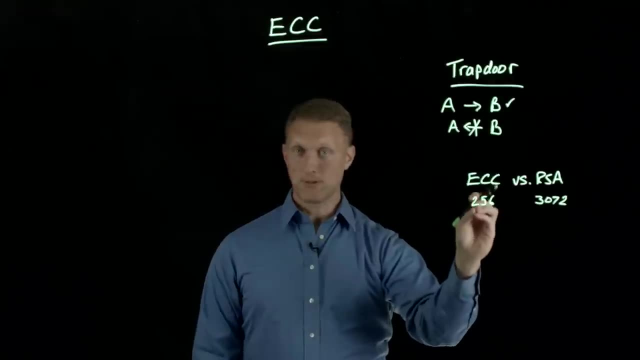 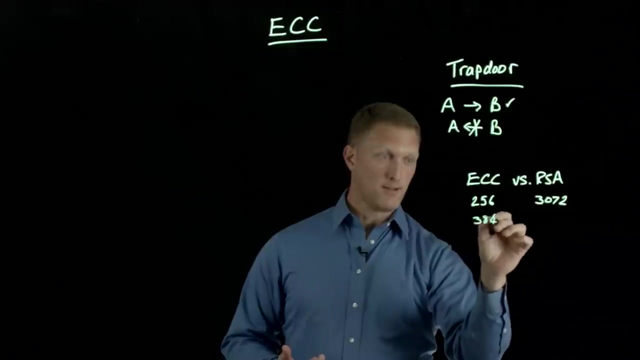 this is one of the reasons that elliptic curve is so much, you know, in demand today. you know, in its comparison to RSA, The key sizes are much, much smaller but you get the same level of security. If we bump this up to 384 bits in ECC, you'd have to go all the way up to 7680 in RSA. 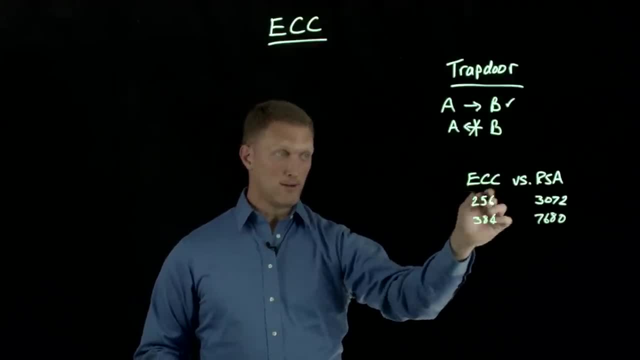 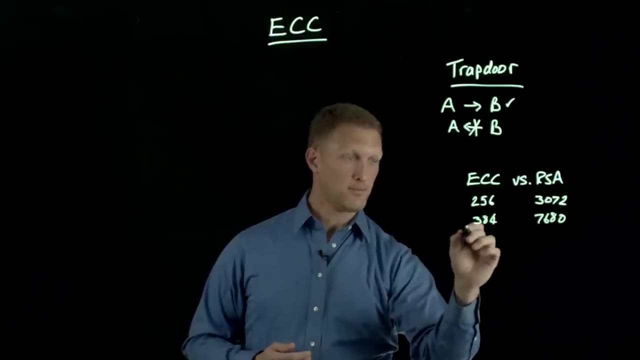 So you can see that, as ECC, you know, keeps this small number of bits, RSA has got to get like huge in order to achieve the same level of security. This right here, I'll put a little TS by that- 384.. 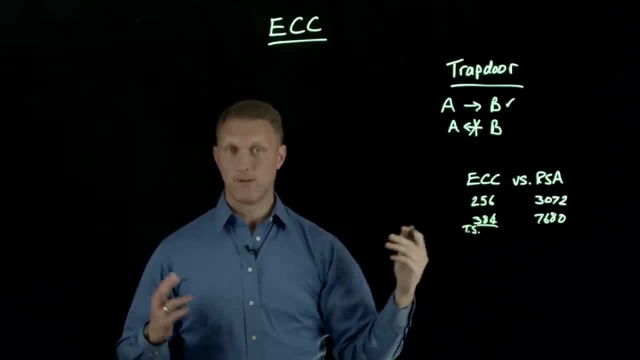 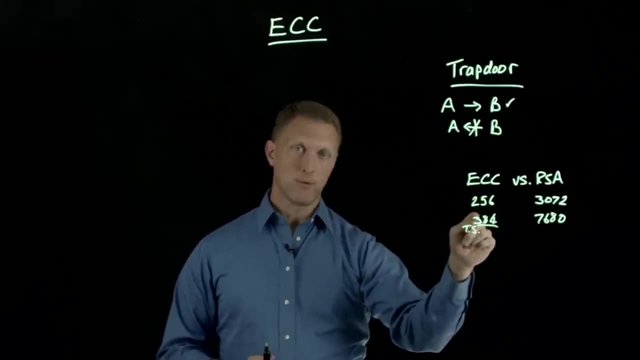 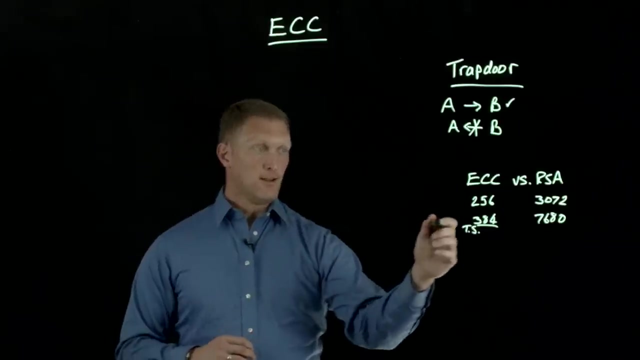 The reason I put that is that's top-secret level information in the US government. NSA and the other government agencies have said that elliptic curve 384-bit keys are strong enough to protect top-secret level information, And so that's a. you know there's no way you would get. 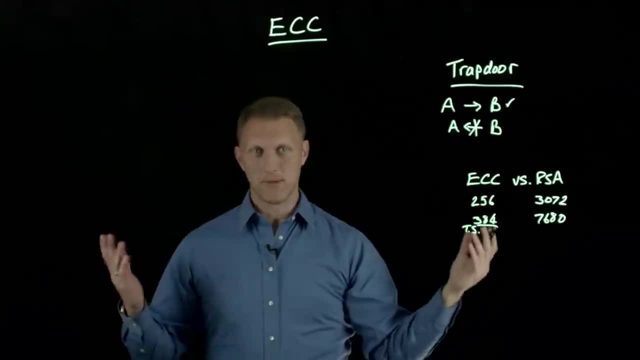 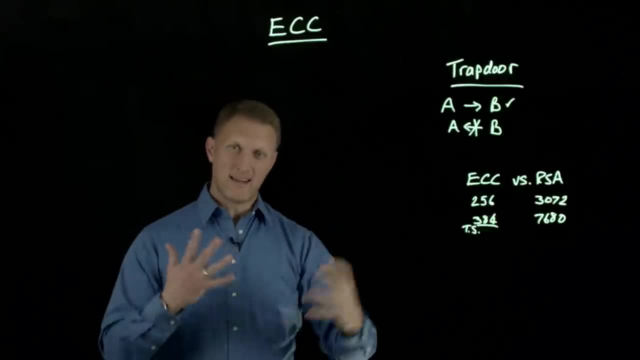 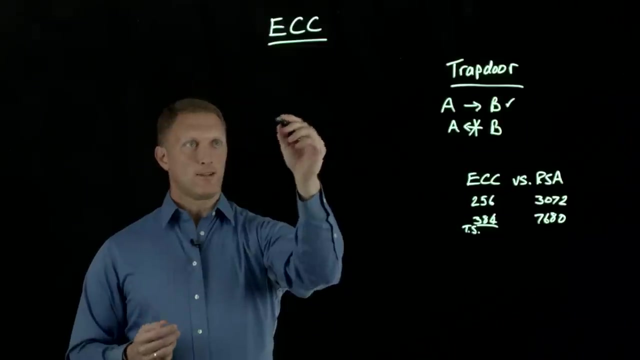 that same level of protection with an RSA key at 384 bits. It's just not going to happen. So anyway, all right. so that's kind of ECC versus RSA. But again, what is ECC? Kind of, how does it work? You know what's the magic behind the curtain, as it were. So what I'm going to do is take 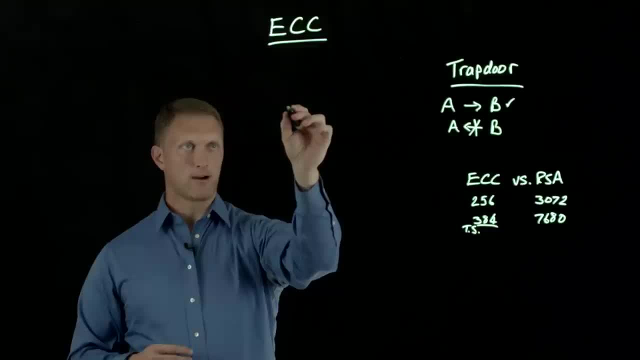 you through kind of a bit of an example of elliptic curve cryptography And I'm going to draw a math graph here, kind of a math function, where this is the X axis and this is the Y axis. All right, So you have this, this is your normal, you know, you remember back to algebra or whatever, and you're. 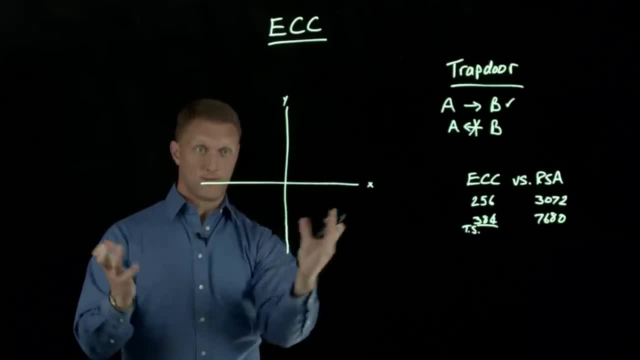 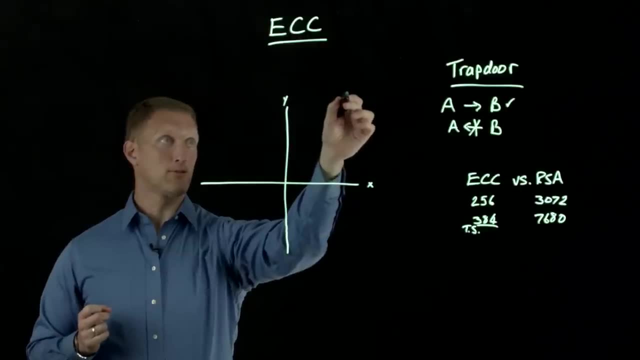 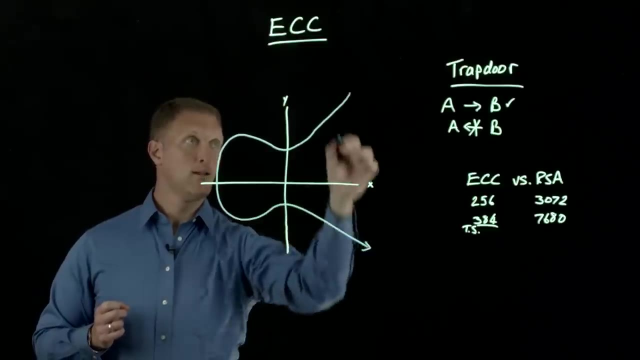 doing your math functions, And so we're going to draw an elliptic curve on this graph, And the elliptic curve has a few interesting characteristics and I'm going to do my best to draw an awesome one right here. So we're going to come like this and that That's not too bad. Okay, A few things that the elliptic curve has is that: 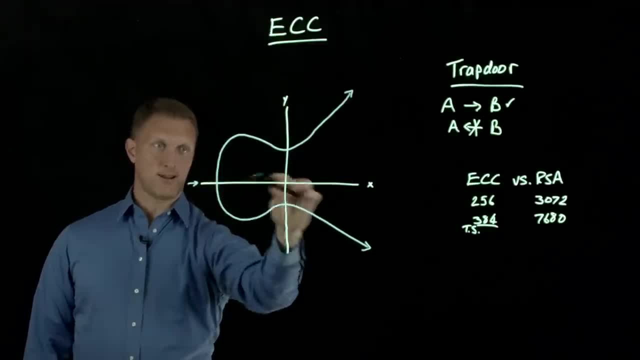 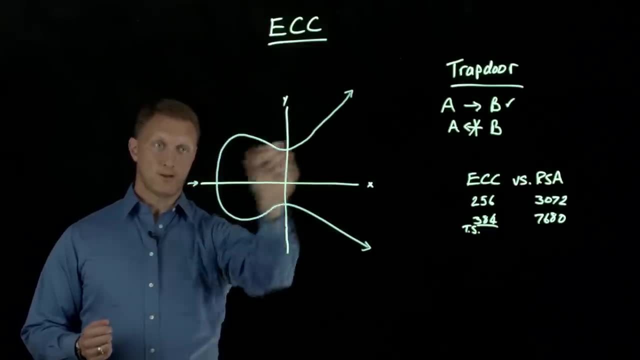 it is symmetric about the X axis. So here's the X axis. It looks the same on top and it's like a mirror image on top and bottom. Symmetric about the X axis. The other thing is that if you draw a straight line, 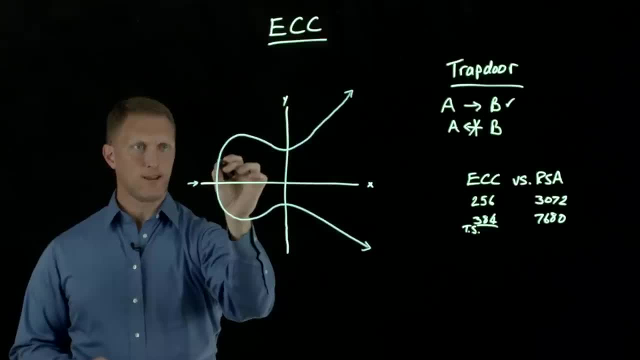 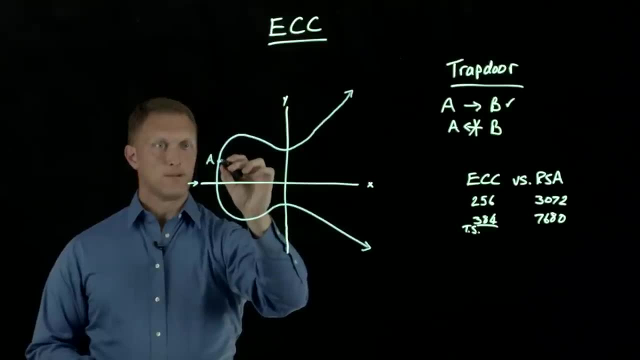 in no more than three points, And so if I were to take a point right here, A and I were going to draw a line through it. it would hit it in another couple of points, And so let me just go ahead and do that. 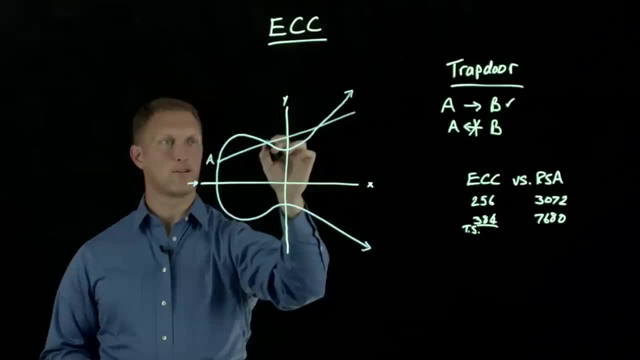 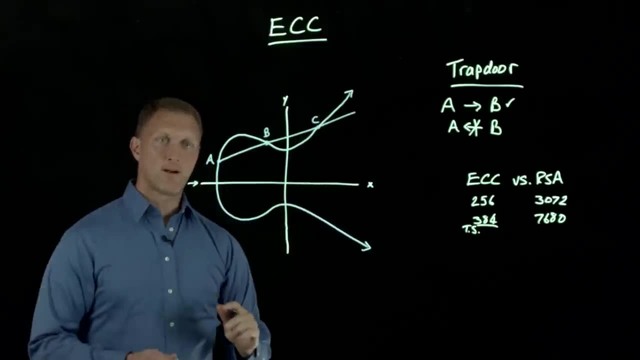 So if I were to draw this line, let's say like that, then it's going to intersect it right here. Let's call that point B, And then- you guessed it, that point is going to be C. Alrighty, So in elliptic. 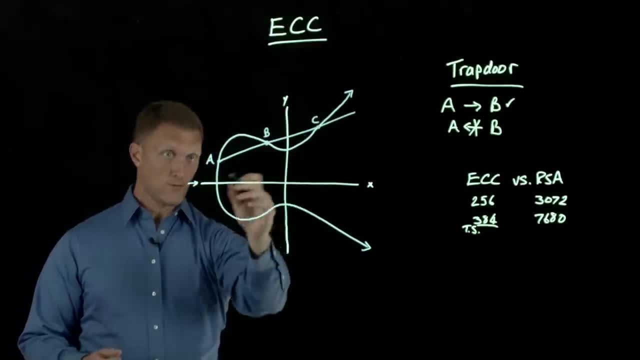 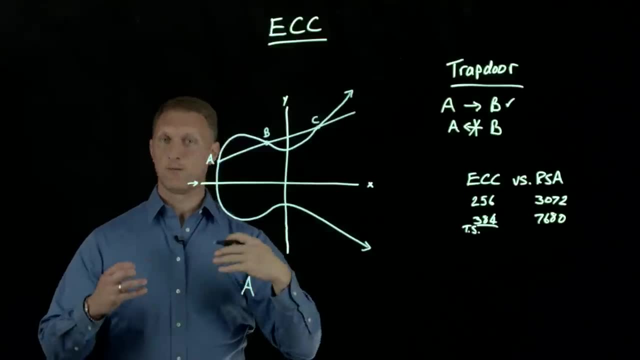 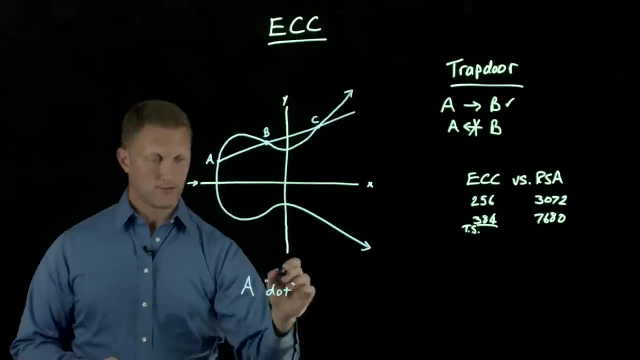 curve cryptography. what happens is you have a curve that's defined by a math function, and then you have a starting point, A, So I'll put A. And then you have this idea of what's called a dot function, So I'll put dot, The dot function, right there. Okay, So A dot, something is going to yield a certain value. 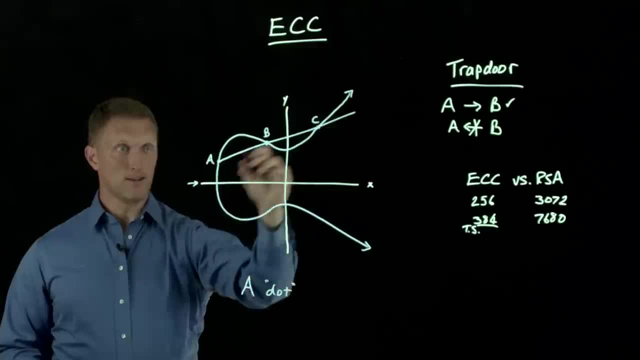 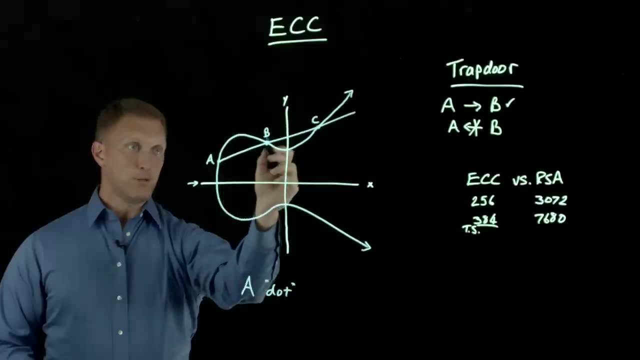 So if you dot A with itself- let's say, I dotted A with itself and it yielded this- essentially- you draw this straight line through the curve and it's going to intersect in these two points. So if I said A dot B, then that would yield C. let's say: 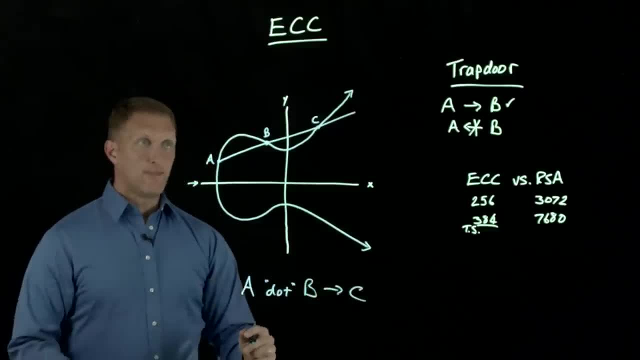 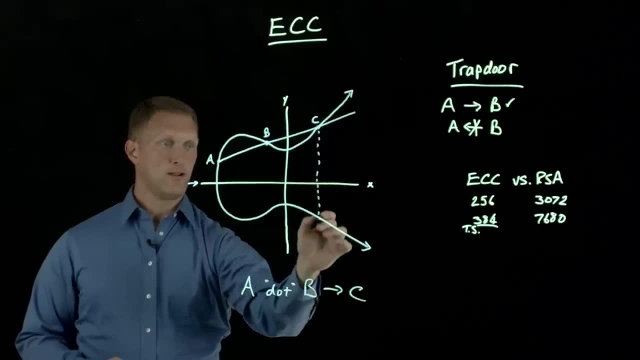 So if I said A dot B, then it yields C And then what you can do is, if you want to do that dot notation again, then you can drop the value from C because of the symmetric property of this curve about the X axis. 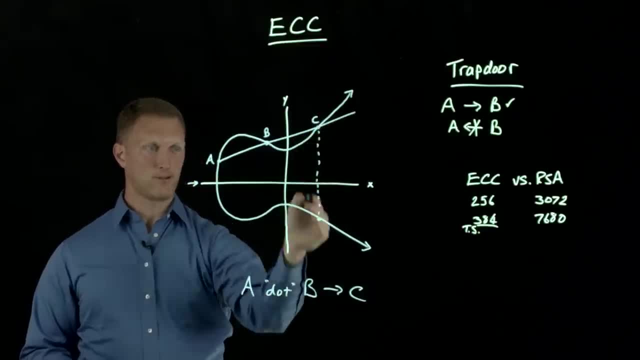 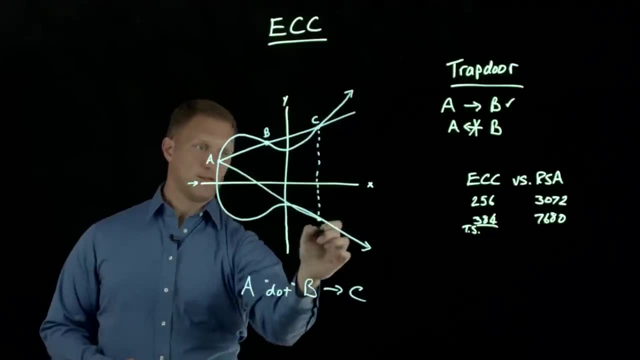 You can drop it down to this: It's the opposite value on the X axis from C, And then you can draw A over to that point, like that. And so let's say that this is a, this is a value D, And then you notice that it intersected again. 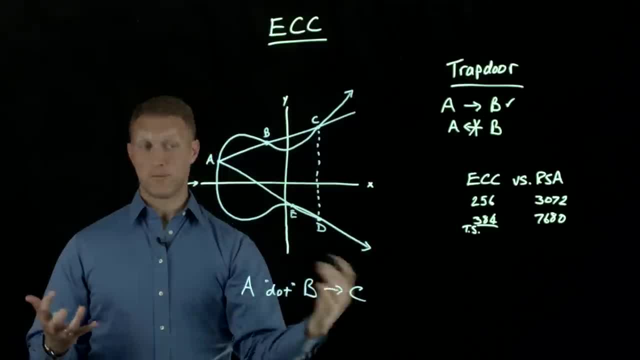 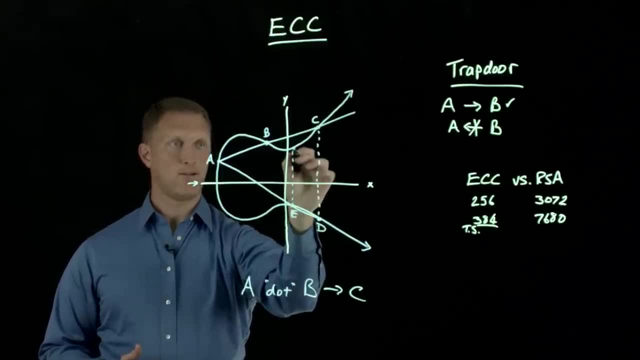 right here. So that's a value E, And then what you can do at that point: you can dot it again, And that's not a very good E. Okay, There's E, So you can dot it again and you can bring that up, and now it's going to intersect it right there. 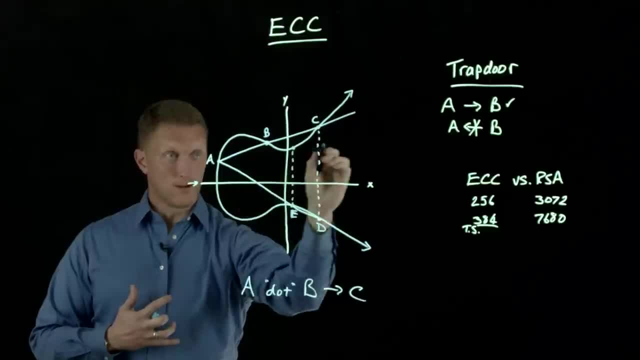 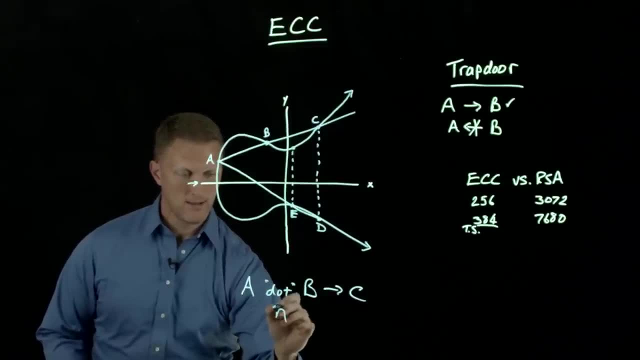 Then you can do, you can start back at A. You can go through that point and then this thing just keeps going over and over And you can dot it a certain number of times And I'll say, I'll say that we'll dot it N number of times. 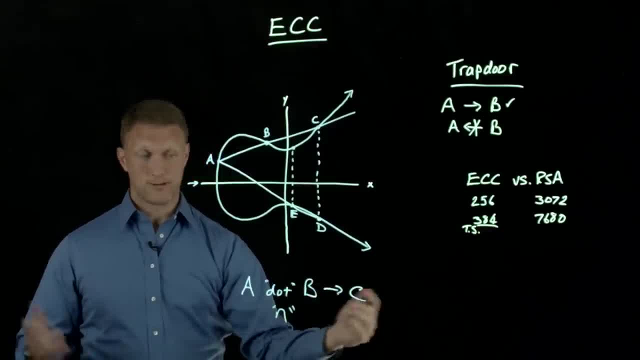 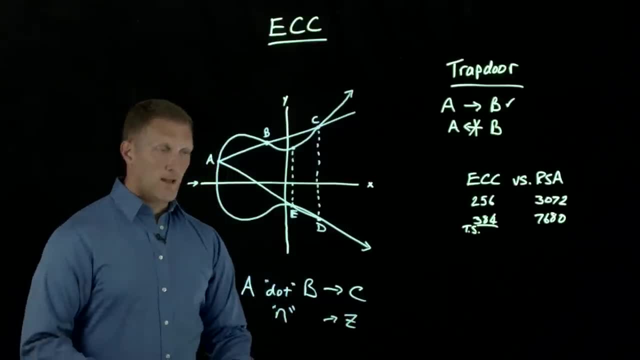 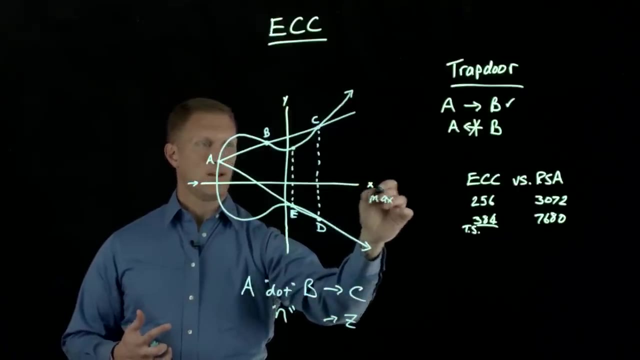 So A dot B or A dot itself, actually N number of times- is going to yield, let's say, a value. I'll call it z, Alrighty. another thing I want to point out is that you have the concept of what we'll call a max value out here and a. 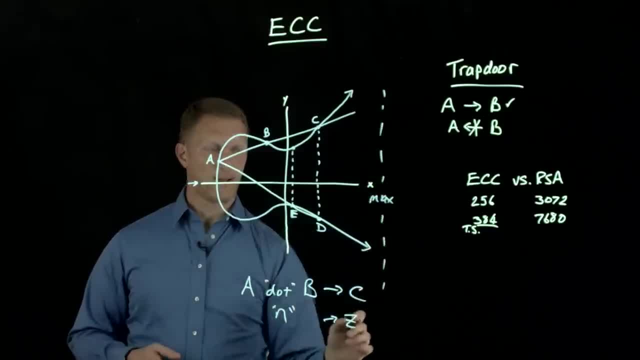 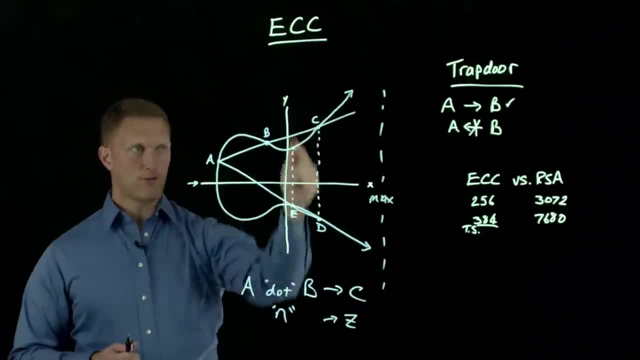 max value on the x-axis. So I'll just put this max line out here and if you can imagine, as you do, this dot function or this dot notation, over and over and over some of these values, that that fall on these on the curve may go like way out. 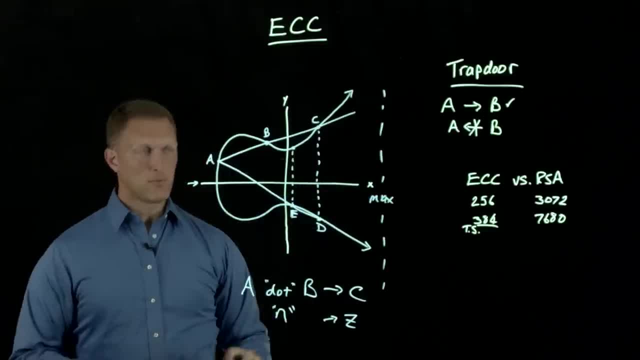 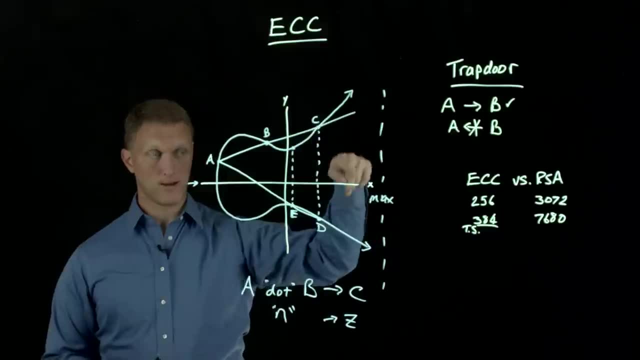 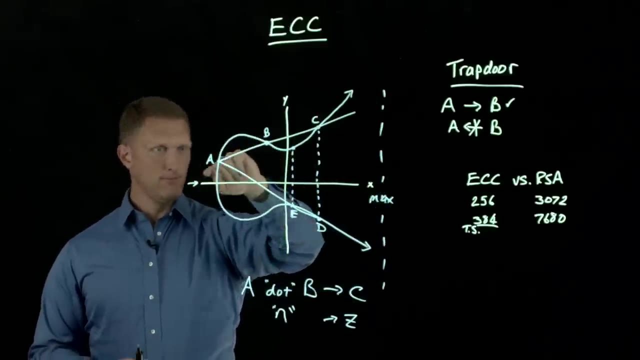 here on the x-axis like way out. you know crazy huge numbers, and so the idea is you can set a max and if you and if the value falls beyond the max, as you're doing this dot notation- then you essentially take the value that would go beyond the max, you bring it back to the beginning and you come over that far and 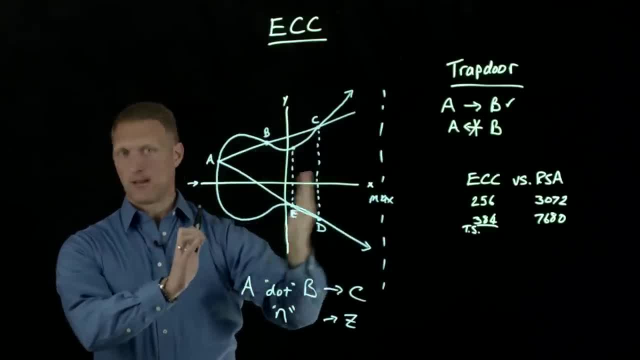 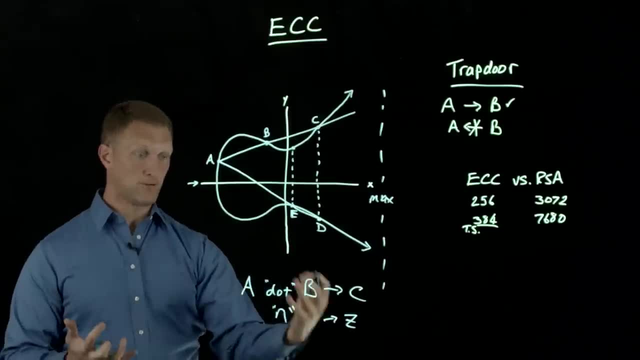 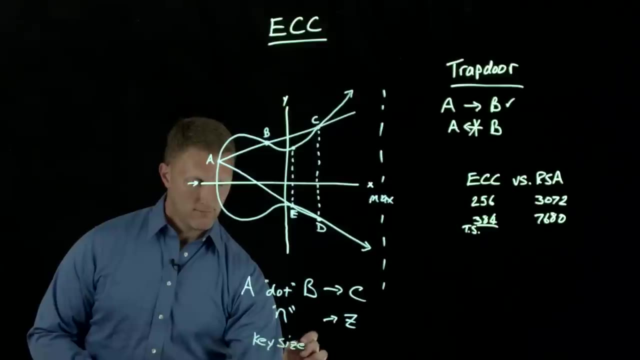 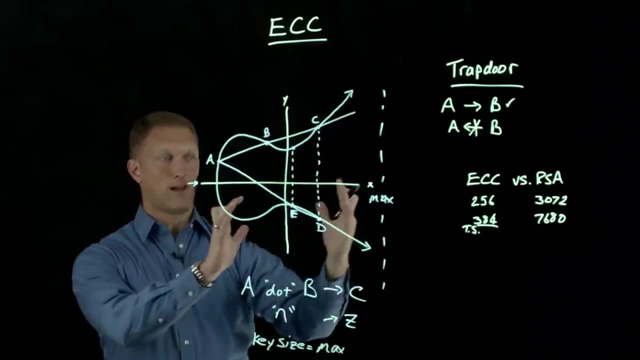 so the the bottom line is you keep everything inside the max value and so the max value when you start talking about private and public keys in in this public key crypto system, the max value is actually the key size. so I'm gonna say key size and a new and an elliptic curve crypto system. you have increased the amount of. 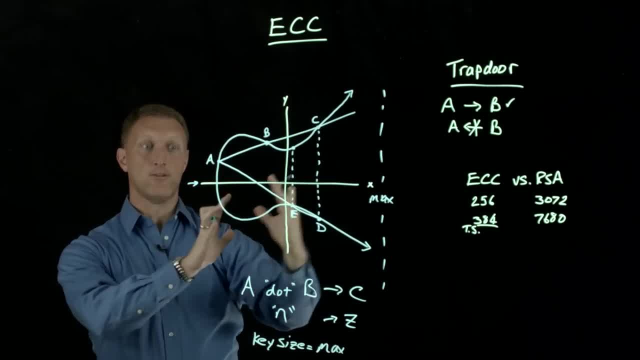 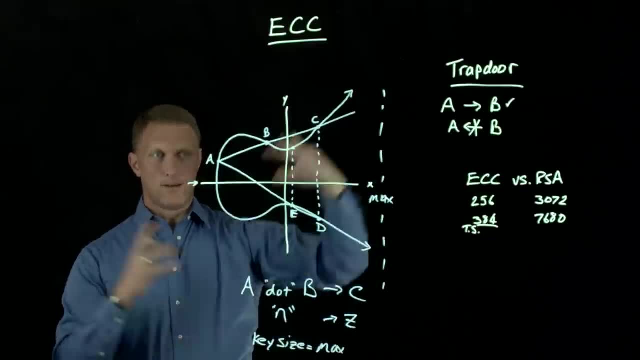 space that you're able to work with now on this curve, you increase the amount of values that would be able to be used as points on this curve. so again, as the max goes out and now you get more points to work with becomes more difficult to you. 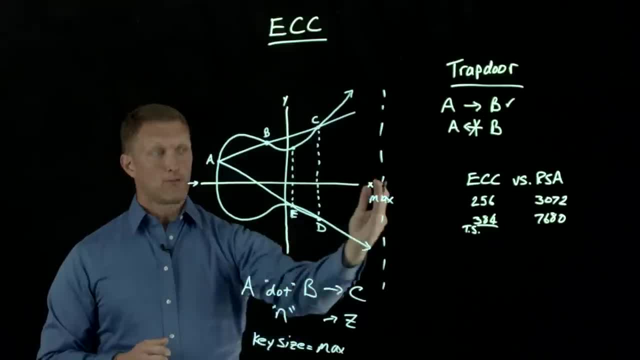 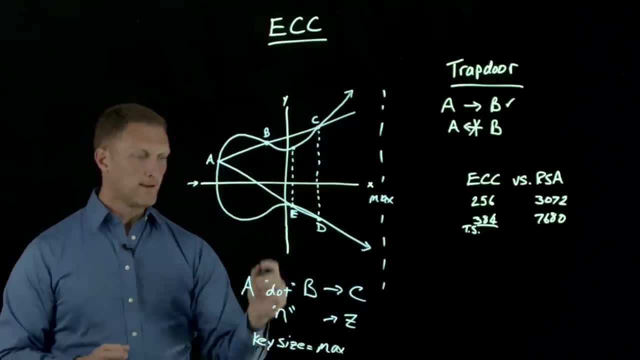 know to undo this thing and try to crack this whole thing, but of course, as max goes out, you've got a, you've got one more numbers to work with, so you've got a crunch through all those numbers as well. so there's a give-and-take, all right. the other thing I was gonna 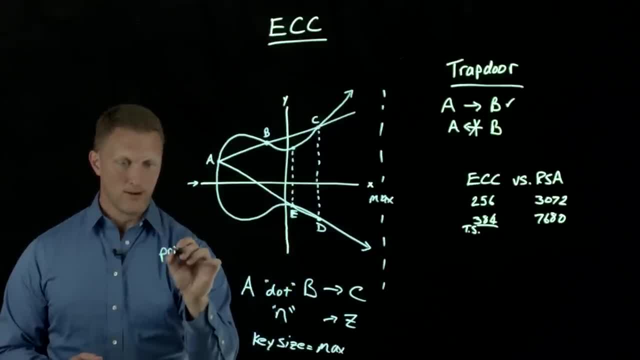 mention is the private key, so I'll put private over here. the private key in an elliptic curve crypto system is actually this, in which is the number, and I'll put dot right here: it's the number of times that you've dot this thing with itself. 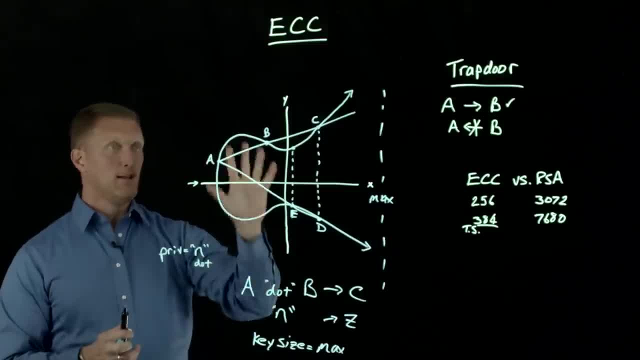 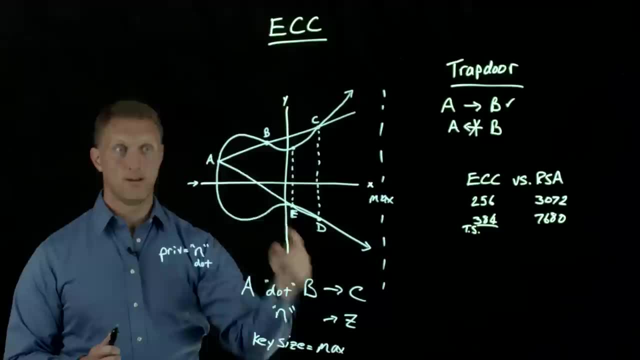 so to kind of to kind of recap a little bit, public or elliptic curve crypto system, you have a, you have a function that's defined, or you have a curve- I'm sorry- that's defined by a math function. you have a starting point a, you have an ending point Z, and then you're gonna dot. 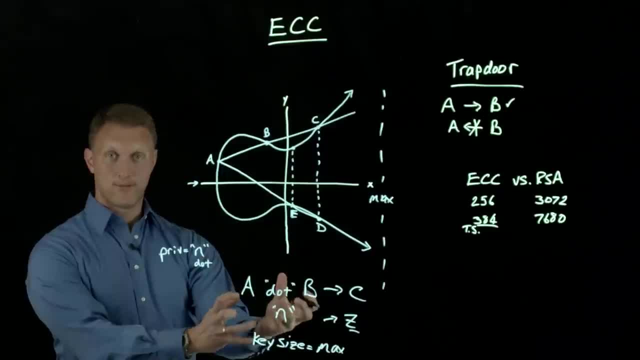 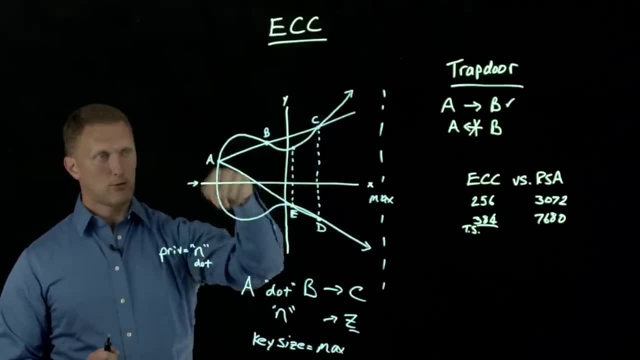 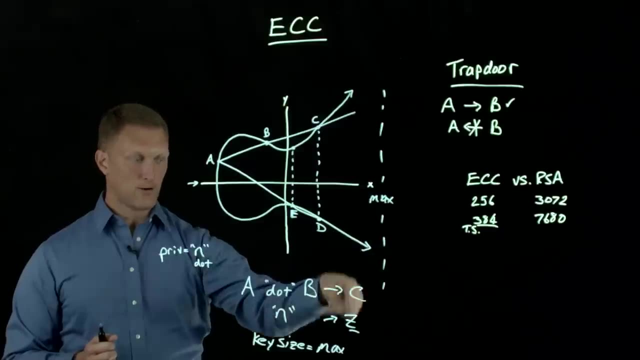 this thing with itself a secret number of times, so an in number of times, and, as it turns out, it's kind of. it's kind of interesting because if, if you are given the actual curve itself, the function that defines this curve, and if you're given the starting point as well as the end point on the 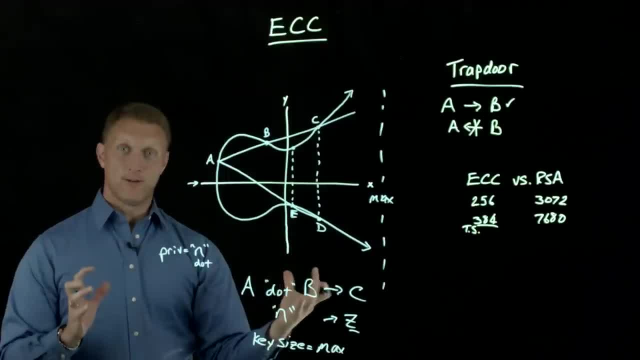 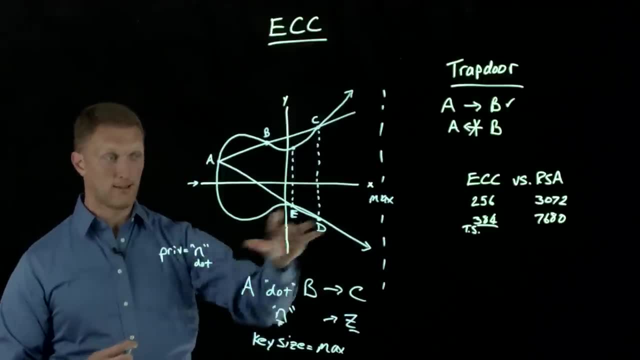 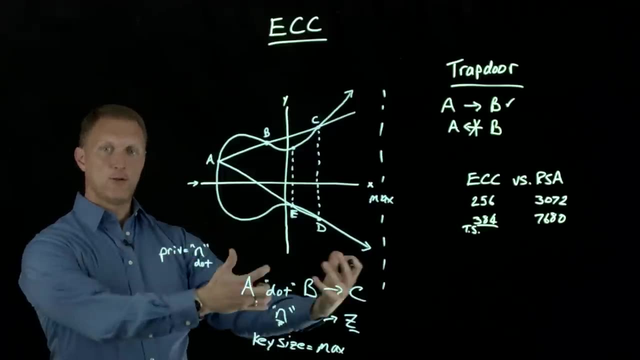 curve this Z point. as it turns out, it's extremely difficult to find out this number for in the, the actual number of times that you dotted the function with itself to get to that point and so that that provides the basis for this trap door function to be able to say, hey, I can give you out public and you know.